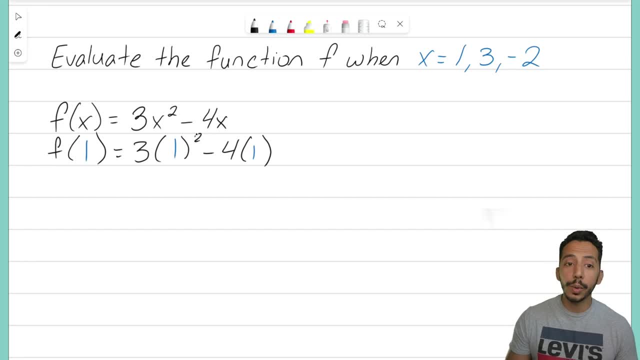 Remember order of operations: 1 squared right, 1 squared is going to be 1.. So I could write this out as: 3 times 1 minus well, 4 times 1 is just 4.. We're getting really close now. Well, let's see. 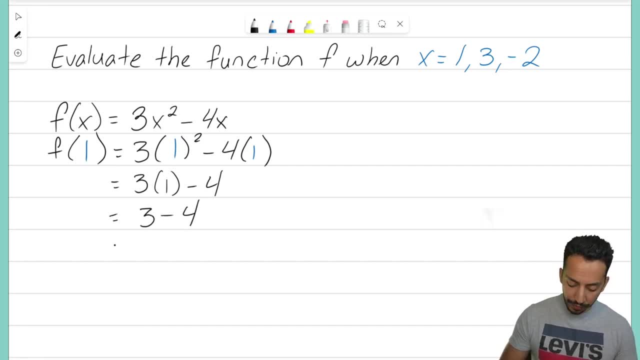 3 times 1 is going to give me 3, and 3 take away 4 ends up equaling negative 1.. So negative 1 is the output when our input is 1.. That right, there is our final answer. Always remember to. 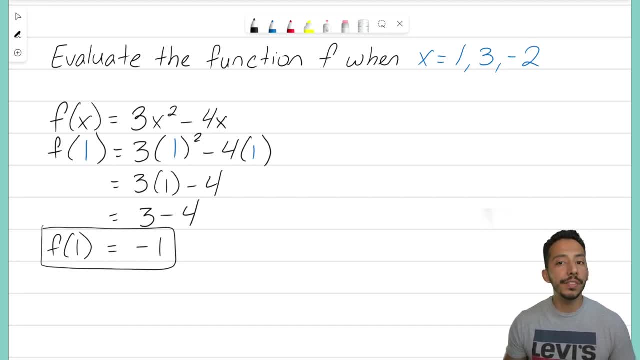 box those answers. That's how you evaluate the function f of x when x equals 1.. Well, the question also says we want to evaluate f when x equals 3.. So we need to now take that same function. I'm going to go. 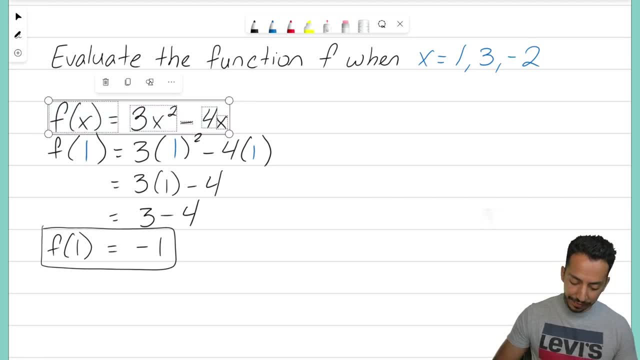 ahead and do this little trick here, because I'm a little lazy. I'm going to highlight that function and I'm going to slide it on over here now. And for f of x again, I'm going to keep that function f, but this time I'm going to change that x value to be 3, because we want to know when. 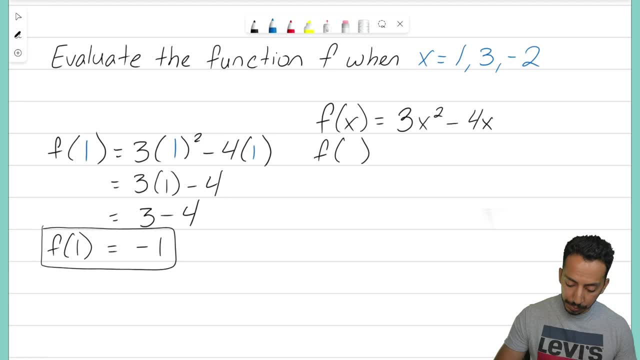 x equals 3, what is our output? So let's plug in a 3.. Everywhere you see an x value, you need to change that to be 3, because we're evaluating the function when x equals 3.. Let's do the same steps. 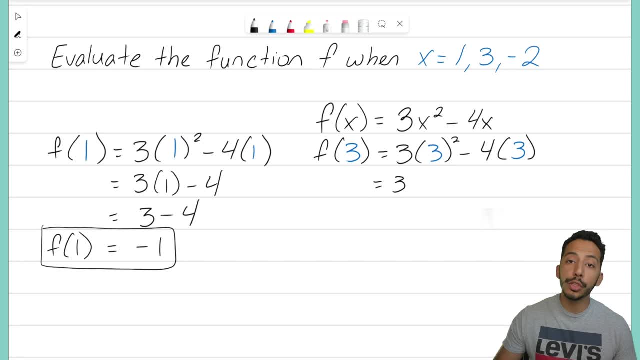 we just did Start with order of operations one more time: 3 squared is going to give us a value of 9.. 4 times 3, well, that equals 12.. We're doing really good, All righty. 3 times 9 is going to. 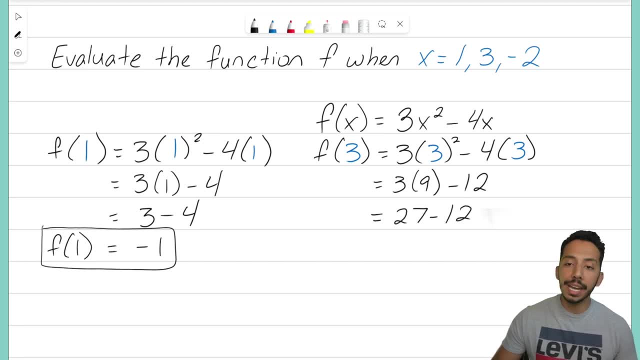 give us a value of 26.. 7. And, last but not least, is: what's 27?? Take away 12.. I believe that's going to give us an answer of 15.. So when we take f, our function, and we input a value of 3, the output ends up being 15.. We have 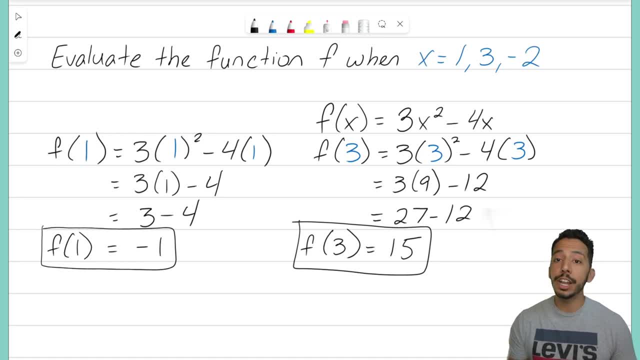 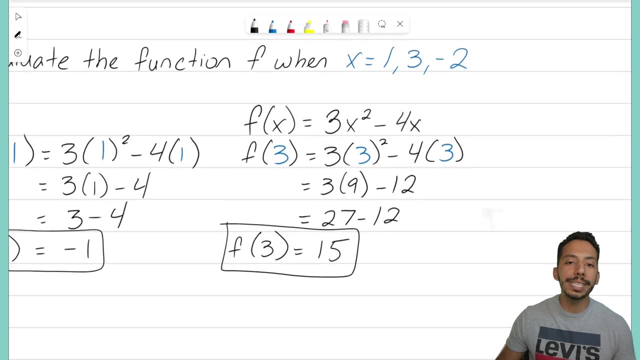 evaluated the function when x equals 3.. And notice two different inputs there. When x is 1, when x is 3, it's giving us two different outputs And that most likely is going to happen Just because of the way our function is. All righty. we got one more input that we want to take.